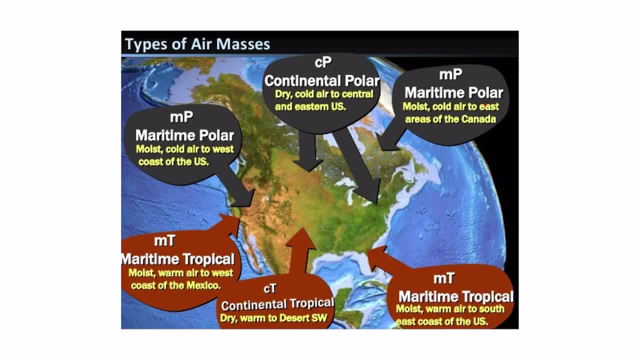 Now, these are the different types of air masses. So we have the polar continental air mass, we have the polar maritime air mass, we have tropical continental and tropical maritime air masses. We also have the arctic and the equatorial air masses. Okay, so here. 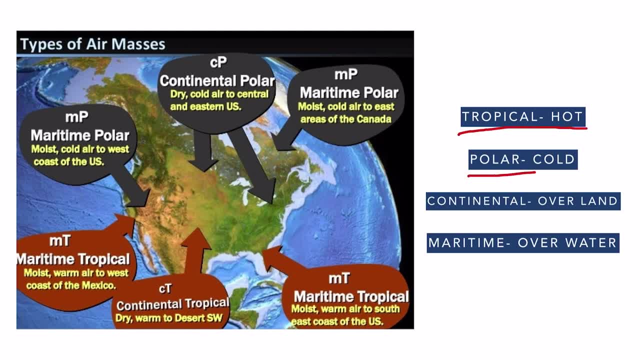 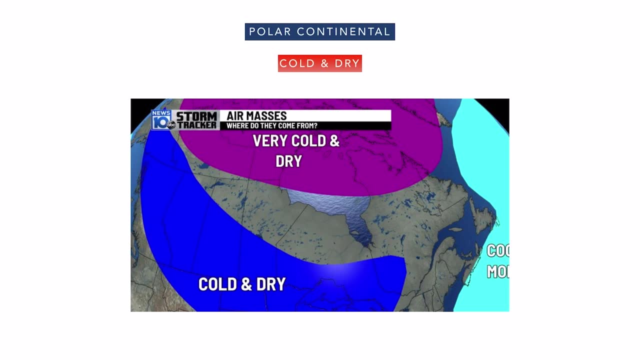 we will be looking at the polar continental air mass. So let's just note that tropical means hot, polar means cold, continental means originated over land and maritime means originated over water. So if you know these four things, you will be able to decode all these air masses. 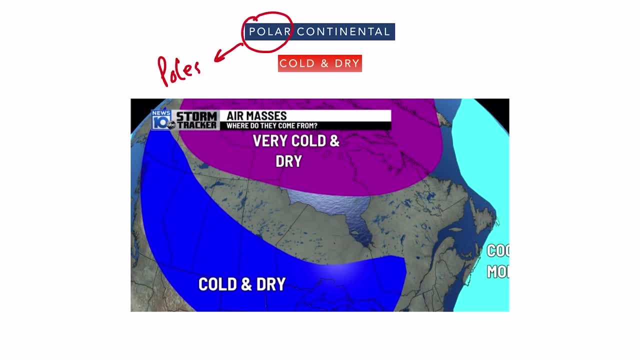 Okay, so the polar continental would mean very cold and over land, As polar means originated around the poles and continental, we saw it, means that originated over land. So this air mass will be dry and because of the poles it will be cold. So polar, continental air. 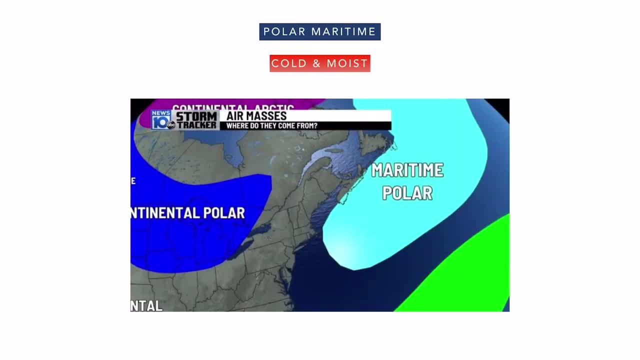 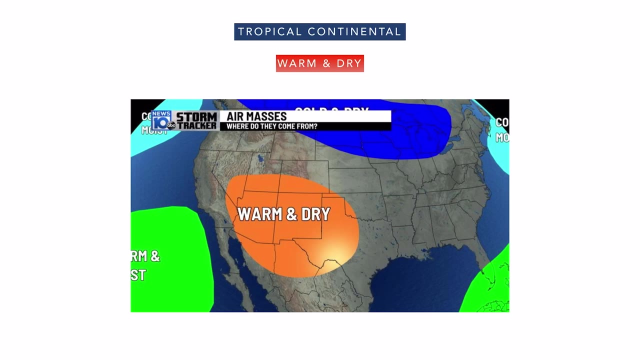 mass is cold and dry. Similarly, polar maritime air mass will be cold and moist because maritime we saw was originated over the water and there is a lot of humidity over water, So that's why it's moist. If we talk about the tropical continental, we see that tropical was warm and continental was. 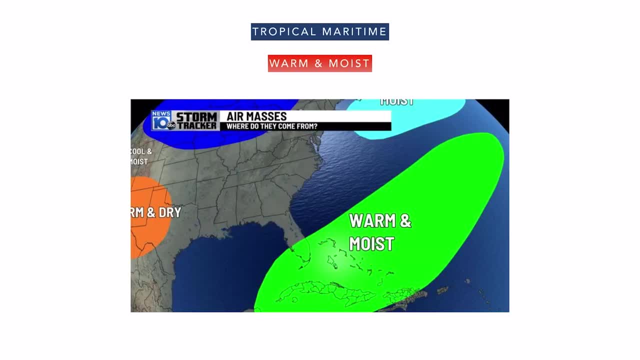 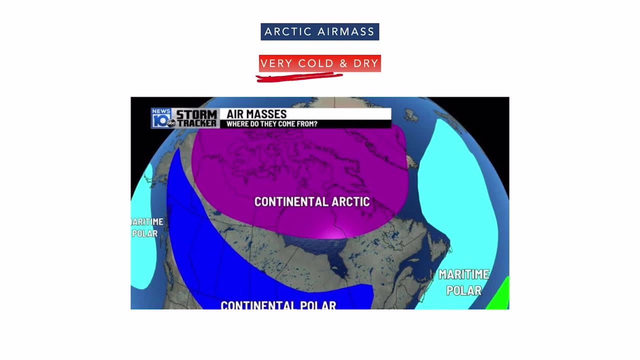 over land. So this air mass will be warm and dry. Similarly, the tropical maritime will be warm and moist, because maritime was over water and water has a lot of humidity, making it moist. Now the arctic air mass has extremely low temperature. The humidity is very less in winter and it increases a bit in the summer. 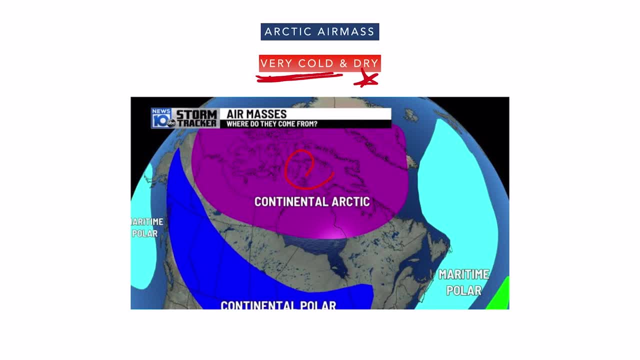 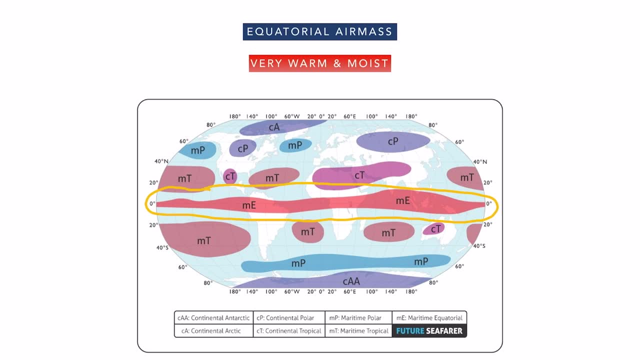 This air mass is originated over the polar regions, So it's over here. The equatorial air mass, as the name suggests, is originated around the equator, with the temperature is very high and the humidity is also a lot, So this air mass is quite warm and moist. 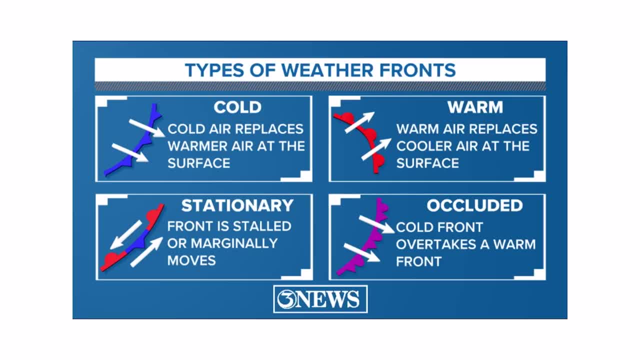 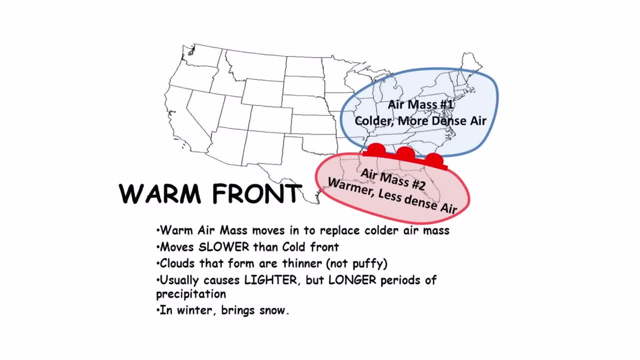 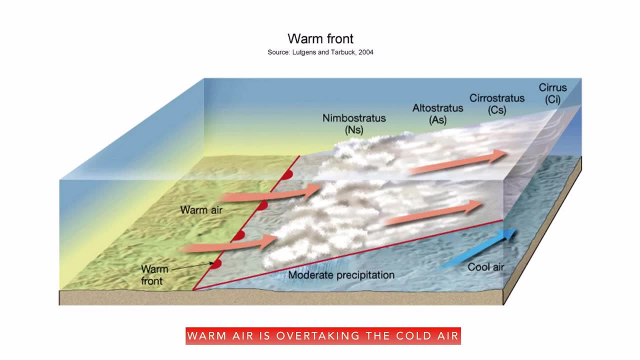 Now let's talk about the fronts. So these are the different type of fronts, and the two main ones are the warm and the cold front. So this is the warm front and this is the cold front. Let's talk about the warm front first. So in a warm front, the warm air is overtaking the cold air. So over here. 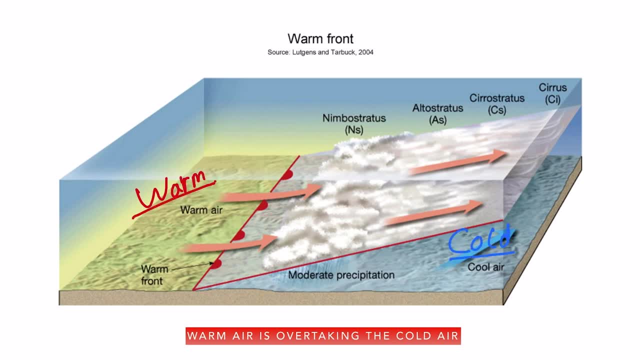 we have the warm air and here is the cold air. So in a warm front the warm air is overtaking the cold air. The warm air is lighter as compared to the cold air, So it glides over the cold air like this. Now in this front we see a lot of stratiform clouds because the slope is not very steep. 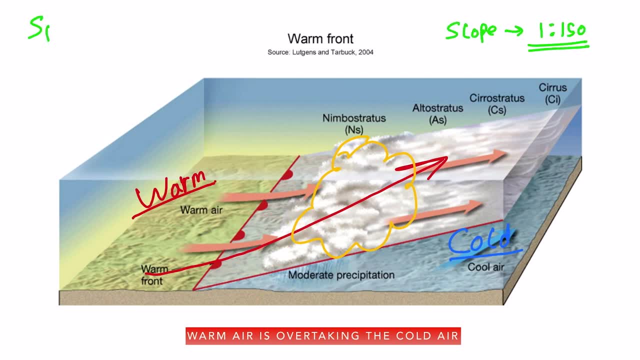 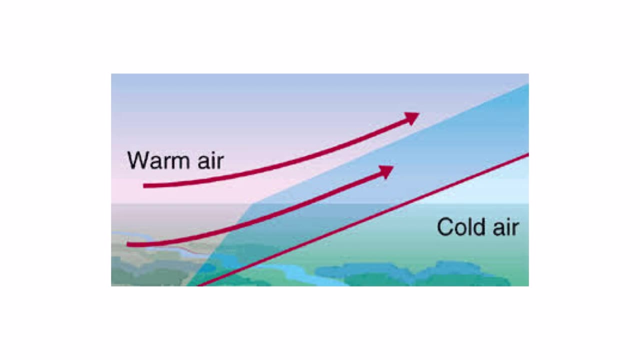 The slope is around 1-150. And a warm front moves very slowly. It's speed is around 10-15 knots. It is so slow because it is very difficult for the warm air to push the cold air, because cold air is. now what does this? 1 is to 150 mean. it means that for every 150 nautical miles the front 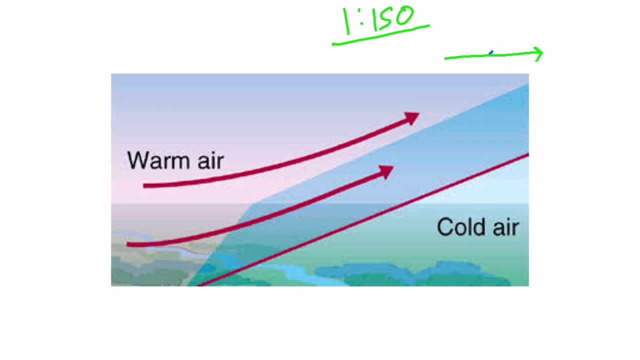 covers horizontally, the air will rise up by one nautical mile, so 150 nautical miles horizontally and one nautical mile vertically, which is quite a shallow slope. so this, you see, is the warm front. it is actually a boundary between the warm air and the cold air. so this is the warm front. 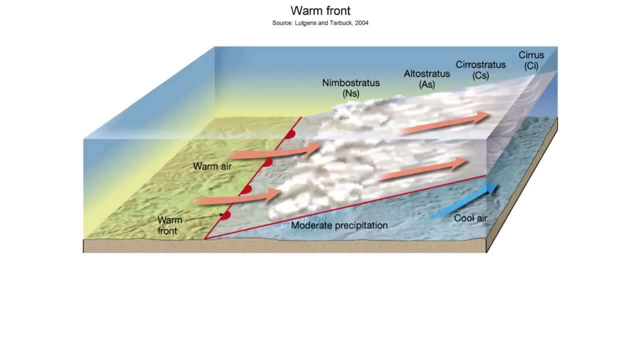 so all this area over here is ahead of the front. so i'll write ahead: this area over here is at the front and all this area is behind the front. i'm specifying it because we'll be talking about the characteristics of all these areas. so in a warm front we experience low. 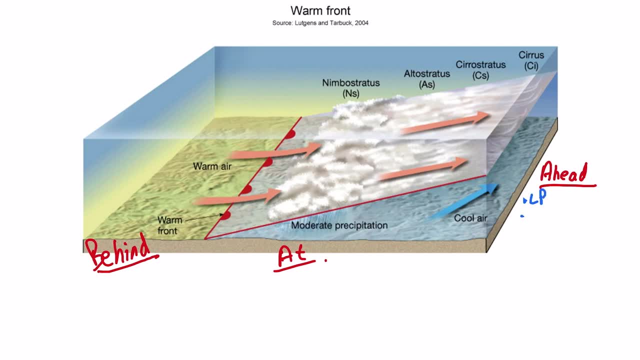 pressure ahead of the front and this low pressure is because of the rising air. so all this rising air gives low pressure on the surface because we saw, whenever there's a low pressure, the air is going up like this. so if this was the ground we experience low pressure over. 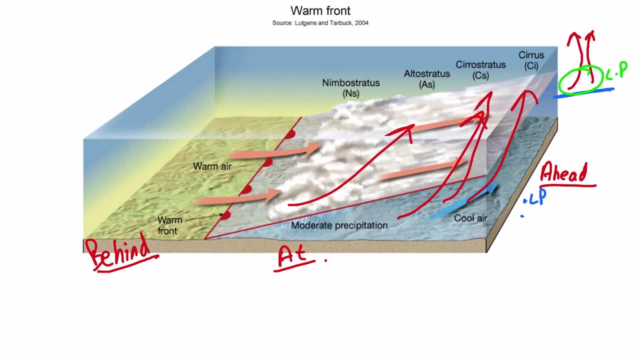 here and the same is happening over here. all this air is rising, so ahead of the front we have low pressure. the winds over here backs and strengthens. we can observe a lot of clouds like stratus, altostratus, cirrostratus and cirrus. the precipitation ahead of warm front is very heavy. 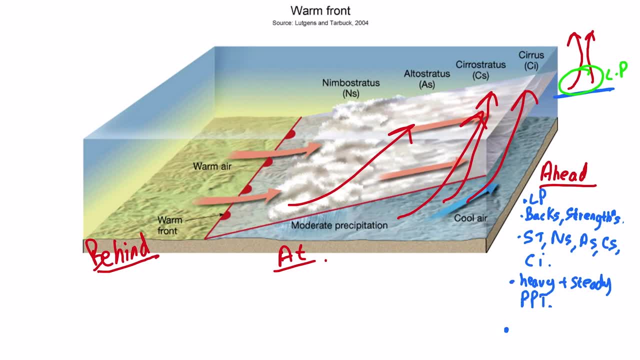 and it's steady, and this steady precipitation gives very poor visibility during rain. and if we talk about the temperature, it's quite less because we saw cool air was ahead of the warm air and we're talking about the area that is ahead of the front. so here we know we have cool air. so the temperature. 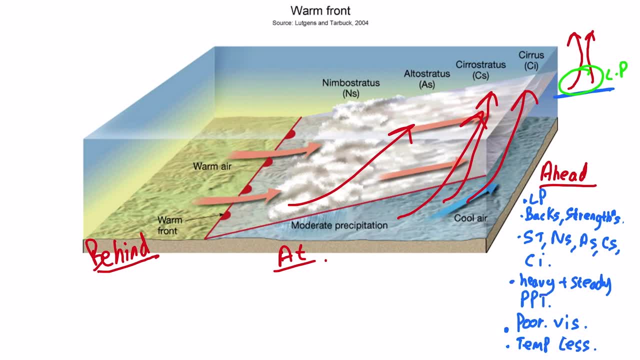 will be less. now let's talk about what happens at a warm front. so at a warm front, when it's passing right above us, we can expect the temperature to rise, because obviously now the warm air is approaching, the pressure over here remains steady, the winds are variable and the clouds that we see over here 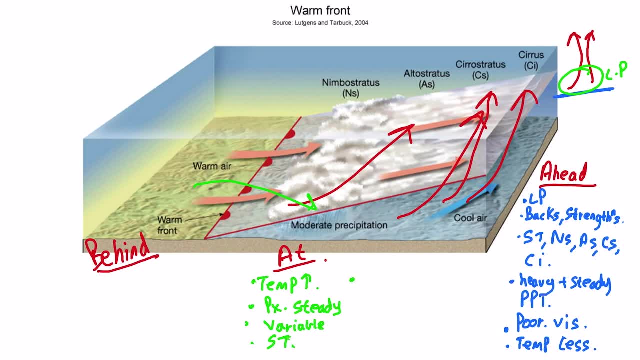 are the stratus clouds and if we talk about the precipitation here, so at a warm front, the rain stops and it starts to rise and we can expect the temperature to rise, because obviously now the warm air is starting to drizzle, the visibility is really, really bad because of fog. now i'll tell you why do we have? 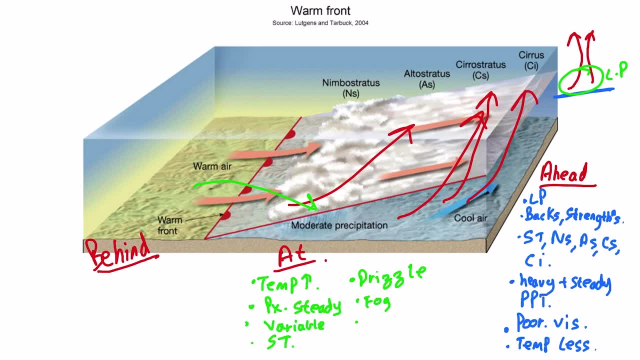 fog. so we just saw that we had a lot of stratus cloud at a warm front, and we know that stratus cloud, when seen on the ground, is nothing but fog. so that's why we have a lot of fog and poor visibility at a warm front now coming behind the warm front after it has passed, so the pressure over here starts to rise. 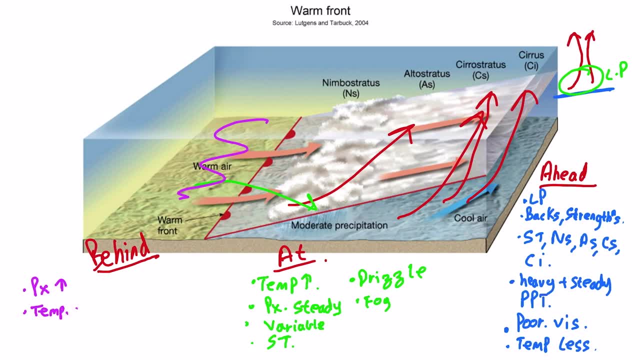 the temperature over here is warm and this is because we had warm air that was coming behind the cold air. so obviously now we're behind the warm front. the warm front has passed us, so that warm air will increase the temperature. the winds over here wear and weakens, and we see. 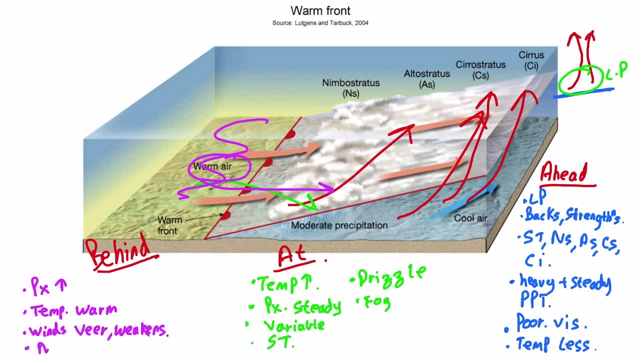 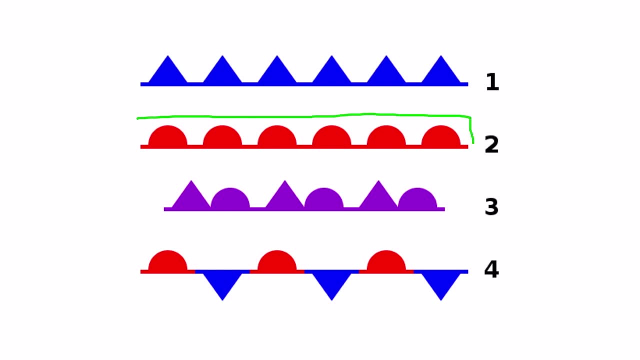 scattered stratocumulus clouds, there is no rain and the visibility is also good over here. a warm front is indicated like this on a surface pressure chart and these semicircles are in the direction of the motion of a warm front. so that means the warm front is moving this way. 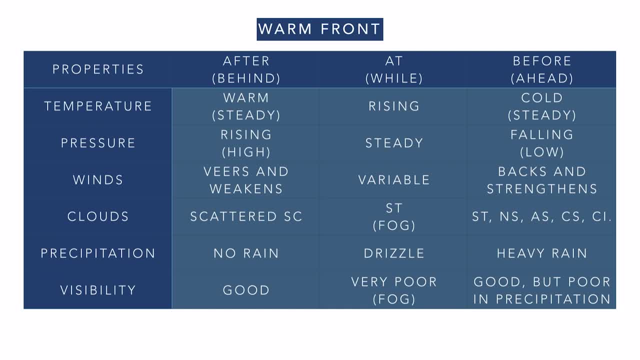 you can refer to this table and learn all these characteristics, because you can be asked anything from this. and also, there's no need to mug up all these if you know the reason why it's happening. i know this table looks very difficult at first, but if you know the proper reason for everything, 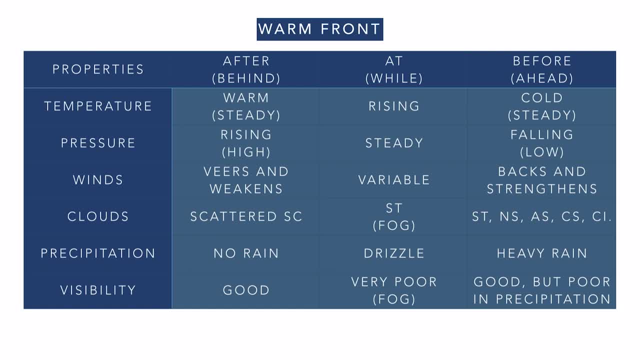 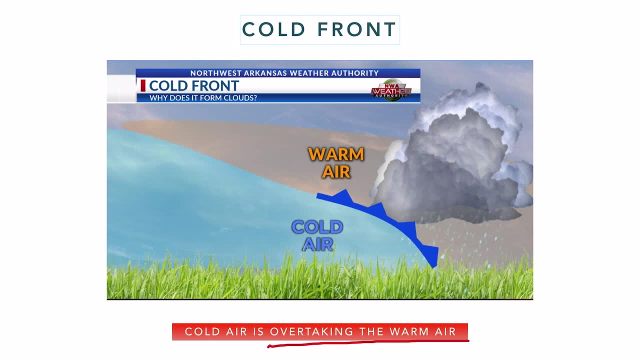 it will be a very easy task to learn it. now let's talk about the cold front. so in a cold front, the cold air is overtaking the warmer air. that's ahead. so we have the warm air over here and the cold air is over here, which is coming behind the warm air, and we know that cold air is heavy. so 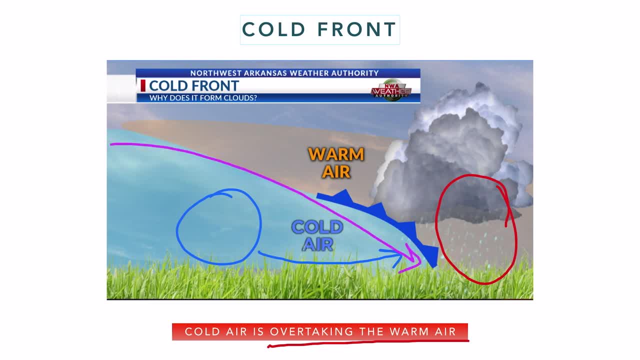 what happens is that the cold air undercuts the warm air, which forces the warm air to start rising. so this is the ground we turn on this liquid. we had warm air over here and suddenly the cold air starts coming and it undercuts the warm air because it's heavy. 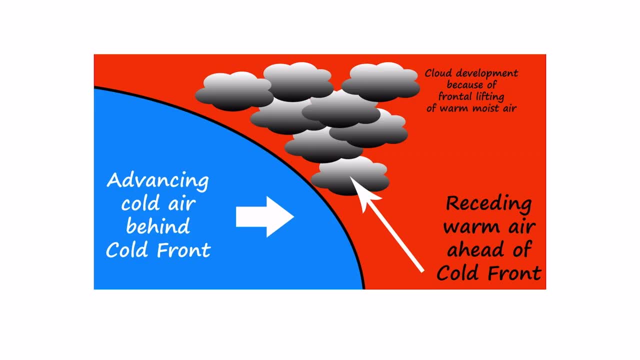 so the warm air starts rising because the cold air is pushing it up. now, in a cold front, very massive clouds of vertical development are observed and this is because the cold air is forcing the warm air to rise. the slope of a cold front is 1: 1 is to 50.. 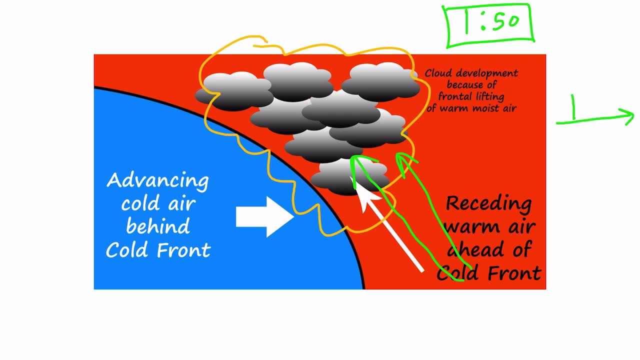 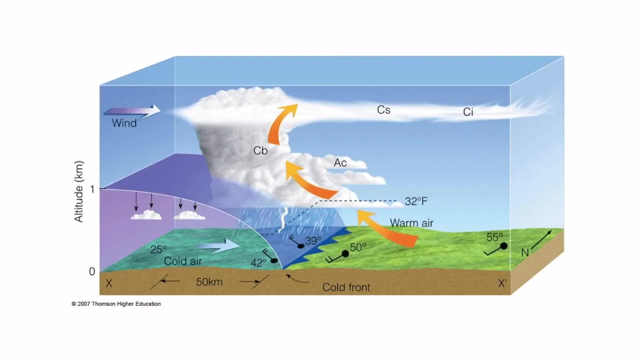 that means 1 nautical miles. it's going ahead. one nautical mile is going up. this shows that the slope of a cold front is very, very steep. the speed of a cold front is about 30 knots, which is two times more than a warm front. now, if we look at this diagram, we can clearly see that the cold air is coming. 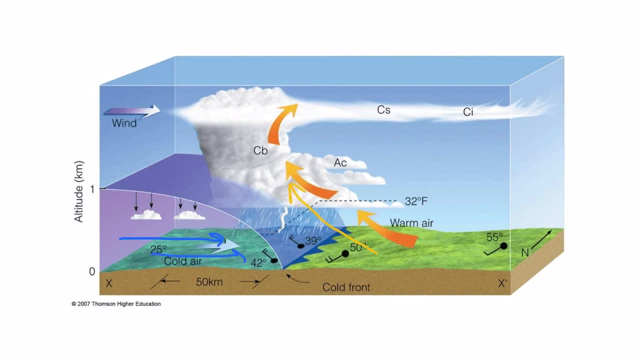 from here and it's pushing the warm air to go up which leads to these clouds of large vertical development. and this is the cold front over here, which is a boundary between the cold and the warm air. in a cold front, we can also observe line squalls. line scores is nothing but a lot of. 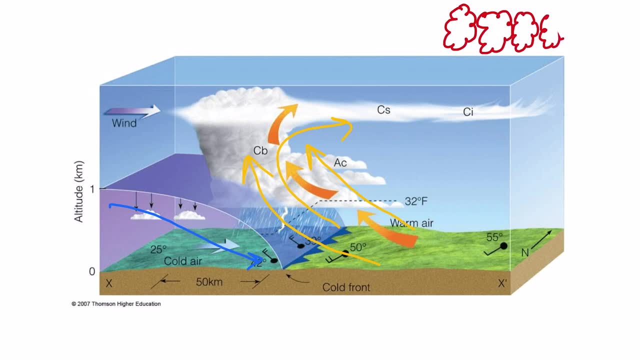 cumulonimbus clouds in one line. so when we see a lot of cb clouds in a single line, we call it a line squall. now again in this front, we'll be talking about the three regions, which is ahead of the front and the front of the front and the front of the front and the front of the front. 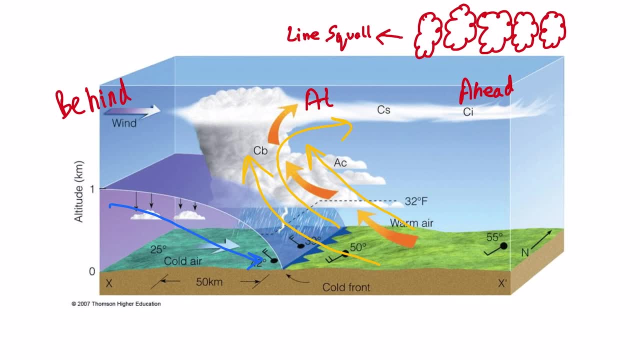 at the front and behind the front. so ahead of a cold front, we again experience low pressure, which is because of the rising air, because here also the warm air is rising and this rising air will again lead to low pressure. so ahead of cold front, we have low pressure, the temperature is warm. 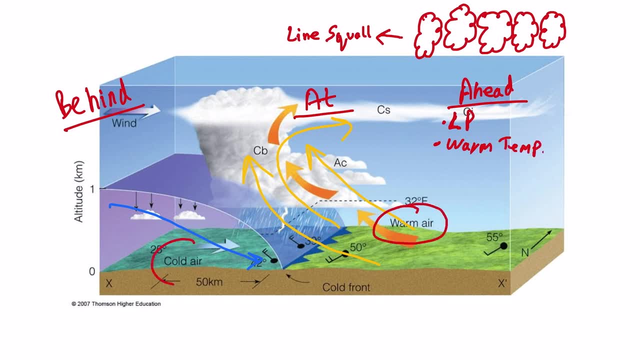 and this was because we had warm air ahead and the cold air was behind it, and since we are ahead of the front, we'll experience warm air which will increase the temperature. the wind over here backs and strengthens. the clouds observed ahead of cold front are cirrus, cirrostratus, cumulonimbus and. 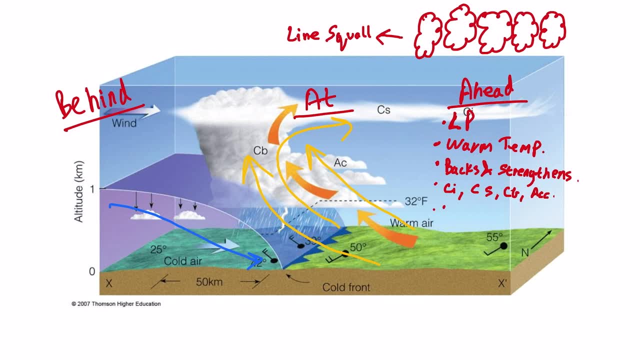 alto cumulus cassilinus clouds: the clouds give heavy precipitation and the visibility is very poor in rain and we can observe lines quals ahead of cold front now at a cold front when it is passing right above us. so when we are over here we can observe. 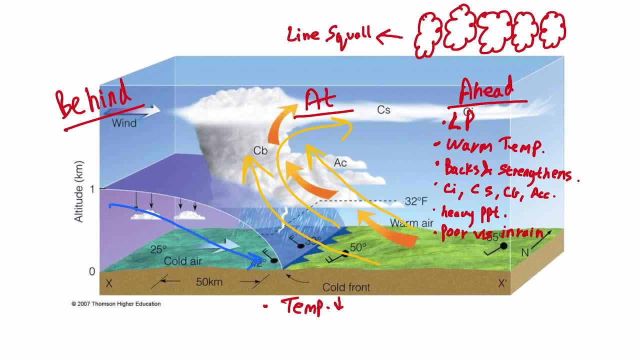 the temperature starting to fall because obviously now the cold air is coming to us, the pressure over here is minimum. and this minimum pressure over here is because we are right under a cb cloud and this area is a low pressure area. also, the winds over here will be gusty and squally. 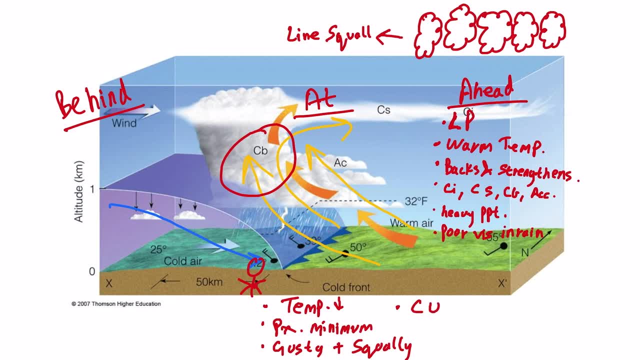 the clouds are either cumulus or cumulonimbus, which gives heavy showers and because of which the visibility is poor. if we talk about the conditions behind a cold front, after it has passed, we observe cold temperatures because now we are in a region where we have cold air. 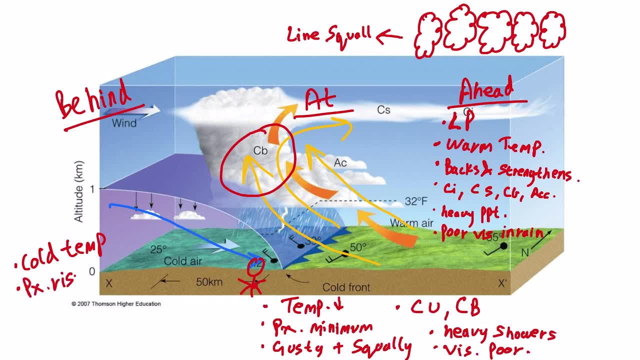 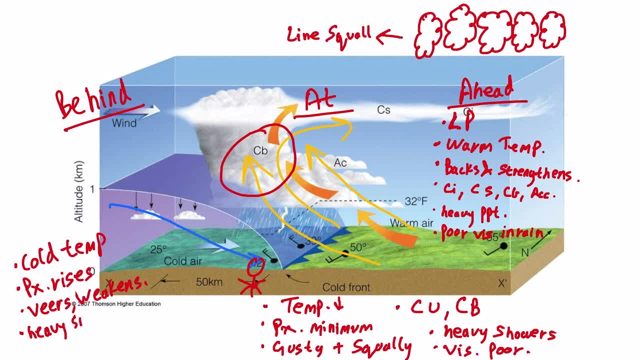 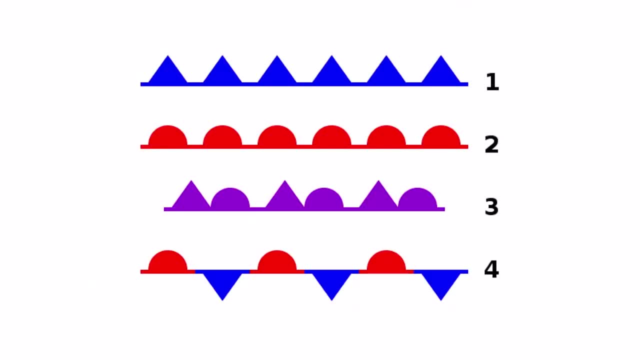 showers clear up and the visibility is bad, initially due to fog, but it improves gradually. on a surface pressure chart, a cold front is indicated like this and again these triangles are in the direction of the movement of the front. so here is the summary table for a cold front. 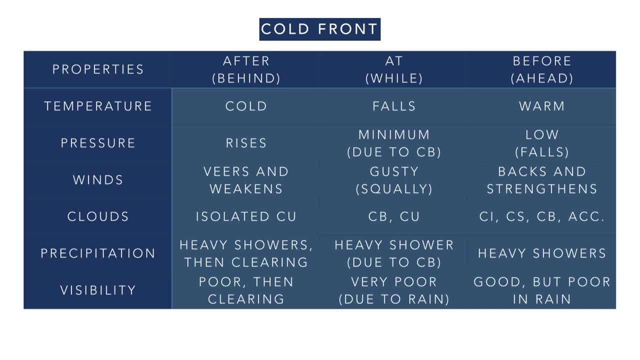 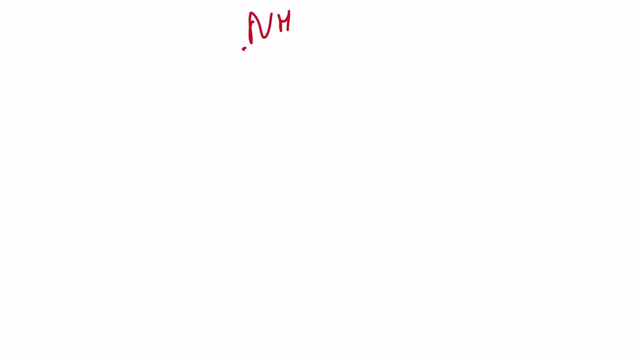 because obviously that diagram was very, very messy. so so see is made so way this. so we know that in the Northern hemisphere, in clockwise and in a low pressure area, the winds move anti-clockwise and we know that when the winds are moving clockwise it's known as wearing, and when the winds are moving anti-clockwise it's. 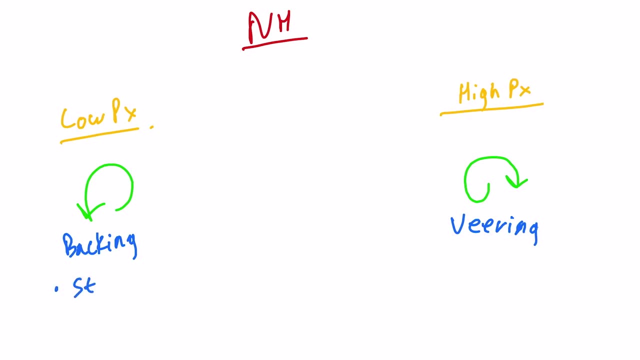 backing. okay, we also know that the winds in a low pressure zone are stronger as compared to the winds of a high pressure zone, and this was because of the isobars. in a low pressure zone, the isobars are very closely packed and in a high pressure zone, the isobars are very far from each other. 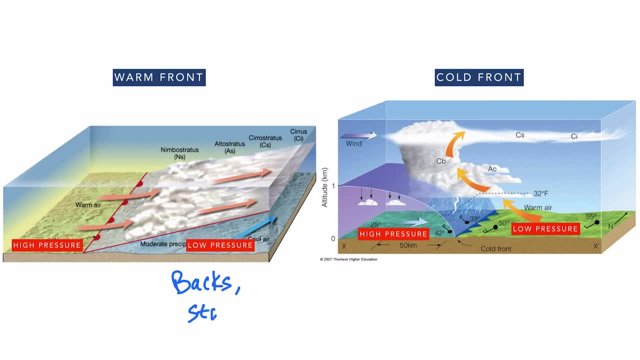 so in the low pressure zones, the winds will be backing and strengthening both for the warm and the cold front, and in the high pressure areas the winds will be wearing and weakening both for the warm and the cold front. so if you know all these reasons, you won't have 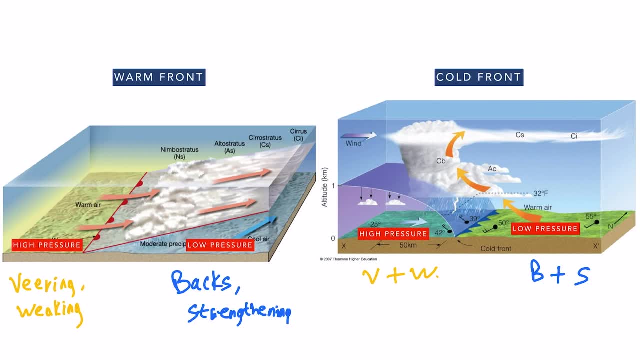 to mug up all the characteristics and you can easily remember everything. now, these are the basics of the isobars and the isobars are very closely packed and in a high pressure zone the isobars are very close to each other. so if you know all these basic differences between both the 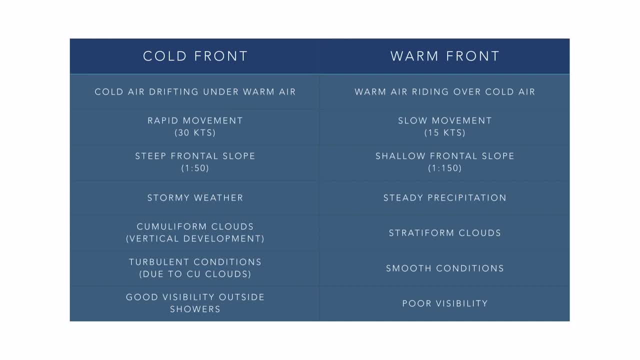 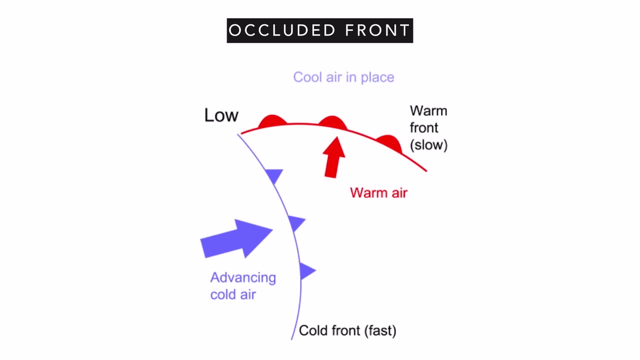 fronts that we've talked about. you can go through this table on your own because we have discussed everything now moving ahead. the next type of fronts are known as occluded fronts, and these fronts form when a cold front coming from behind catches up a warm front that is ahead. this is 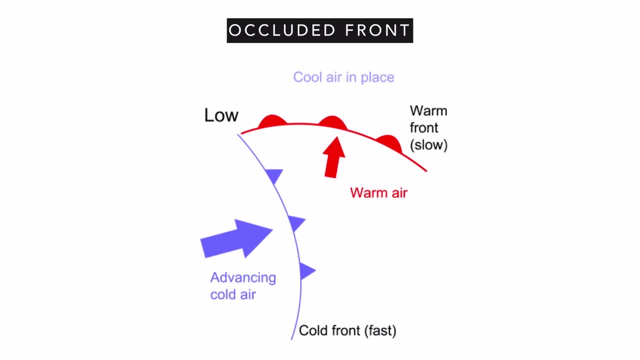 quite possible, because we know that a cold front moves at twice the speed of a warm front. so in this diagram, this is a cold front and this is a warm front, and this is a cold front and this is a cold front, and what we see over here is that the cold front is approaching and is catching up to 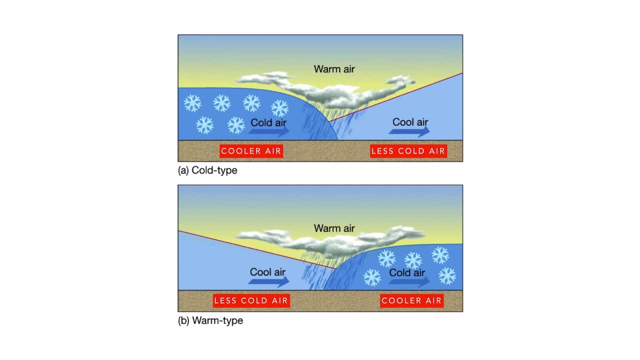 this warm front. now there are two types of occluded fronts: a cold occlusion and a warm occlusion. both of these are when a cold front catches up a warm front. so cold occlusion is seen when a very cold air mass is replacing the less cold air that is ahead and warm air is seen above. 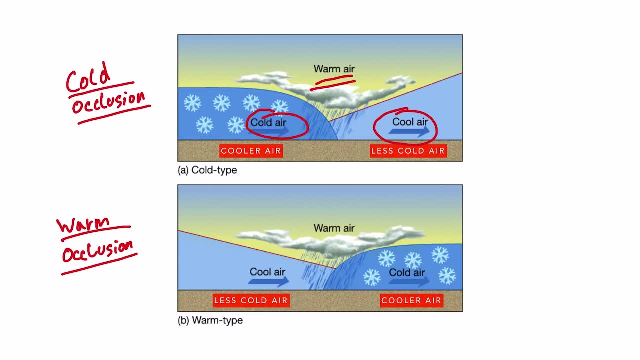 this is common in winters and it's known as the western disturbance. you should watch the indian climatology video on winter season to know about the western disturbances, just to give an idea about what's our western disturbance. so in the winter season we already have the cool air in india and colder air from the mediterranean sea. 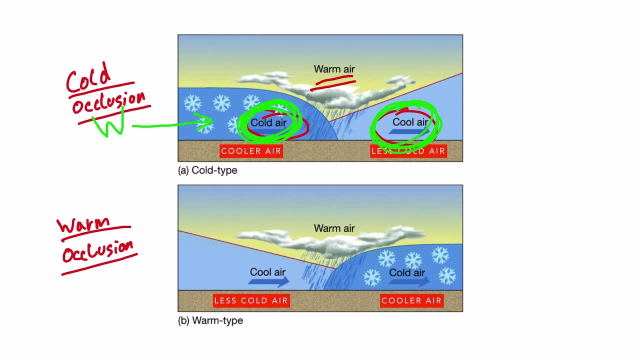 or we can say that the colder air from west comes and replaces the already cold air that was in india, and this results in a cold occlusion, and this is what it looks like. so we have cold air ahead, we have colder air behind and the warm air is pushed up. now a warm occlusion is seen when 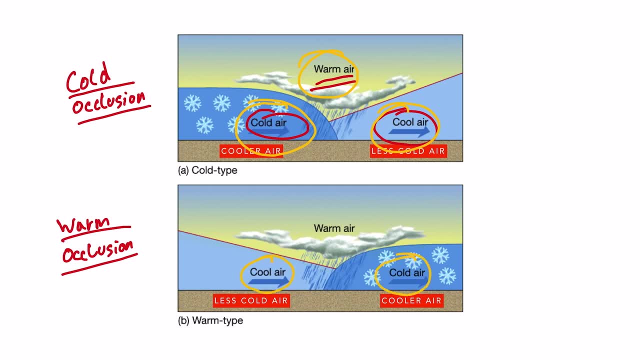 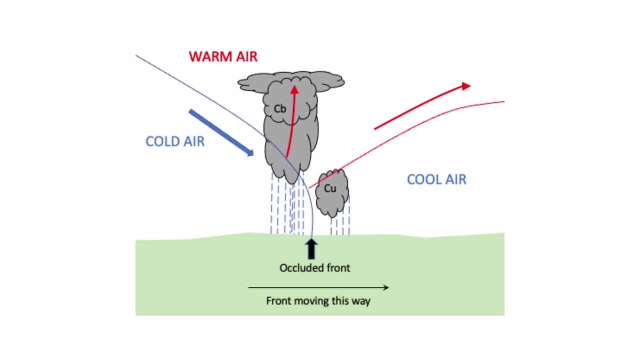 less cold air is replacing the colder air that is ahead, and warm air is again pushed up. warm occlusions are not very common in india. in occluded fronts the weather is quite intense and we observe embedded cumulonimbus clouds. so the cumulonimbus cloud is embedded here like this: between the two cold air masses, one is over. 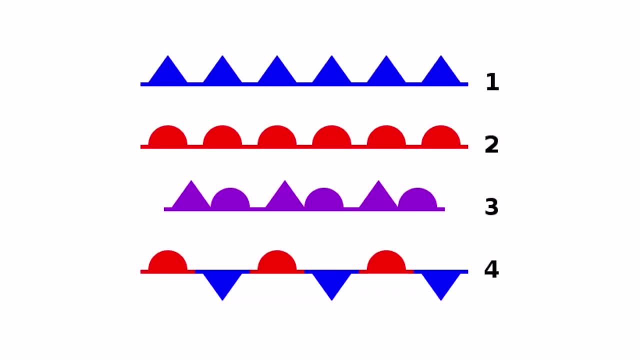 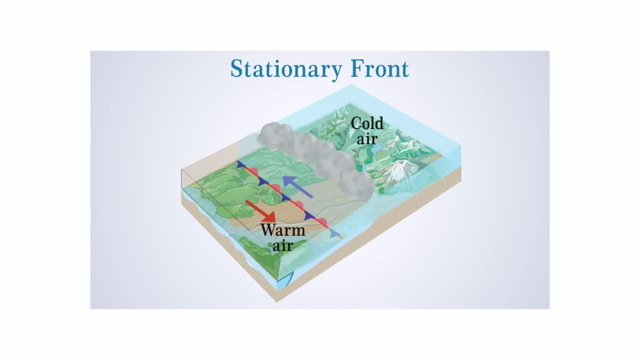 here and the other is over here. now, on a surface pressure chart, an occluded front is indicated like this: it has both the cold and the warm front, and this is because it's a combination of both the fronts now moving ahead. next we'll talk about a stationary front. so a stationary front has 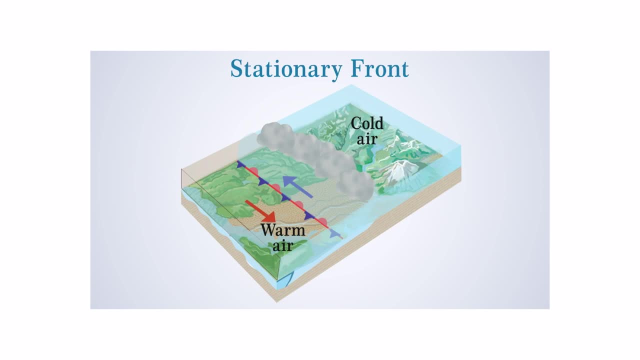 two different air masses on both sides, so the warm air and the cold air are embedded here like this is over here, the cold air is over here, and thus this is a stationary front, which is the boundary between warm and cold air masses. the winds in a stationary front blow parallel to the front, and